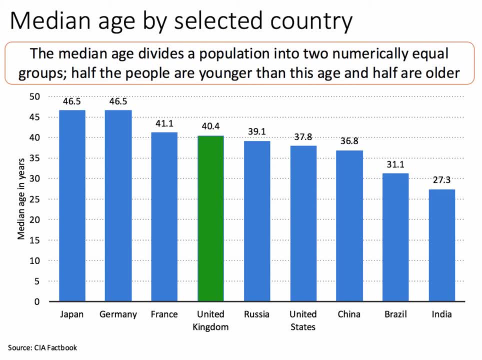 of the chart, 40.4 as a median age. Of course, that's the middle value in a numerical group. Some countries have a significantly older population, and two important ones to mention are Japan and Germany, whereas other countries, particularly in emerging developing countries, have a significantly younger. 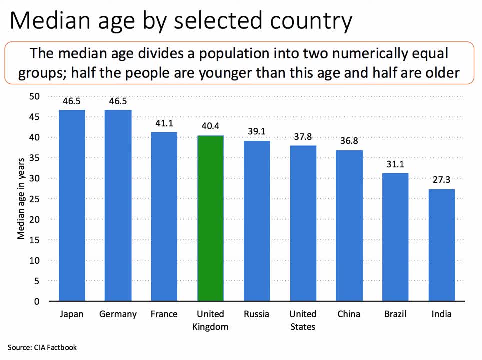 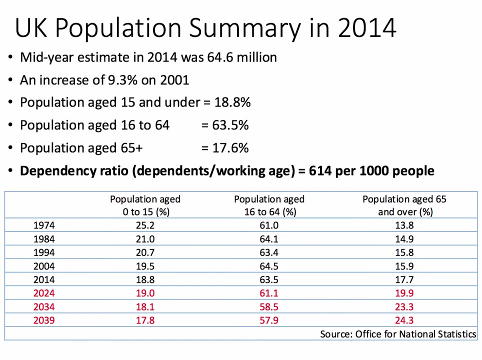 population, including, for example, Brazil and India. Worth noting here, of course, the difference in the median age between India- 27.3, and China- 36.8.. China's population is aging quite rapidly. Indeed, the age dependency ratio, for old people in particular, is likely to rise significantly in the next few years. So 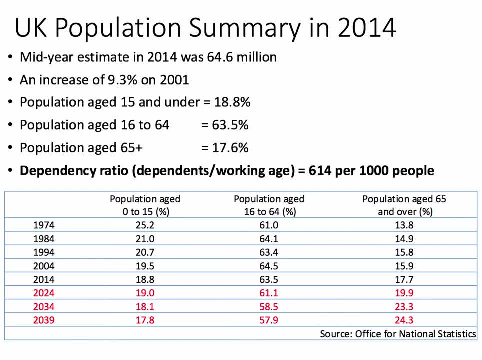 here's a summary of the UK population, which includes the age dependency ratio. The age dependency ratio, which is dependents divided by the working age population, was 614 per thousand people in 2014.. Note in the table below that the population aged 65 and over, express as a percentage of the total population, is: 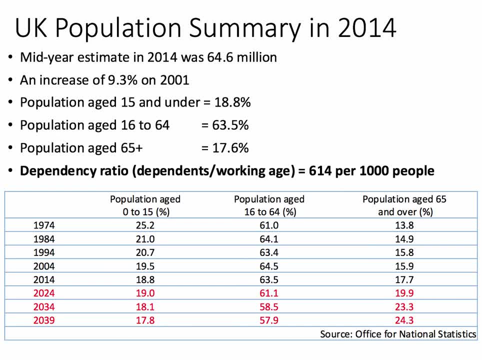 forecast to nearly double from 1974 through to 2039.. By the 2030s, around a quarter of the UK population will be aged over 65.. Of course, our interpretations and understanding of what retirement will mean may well have changed significantly by the time we get there. So let's take a look at this chart. 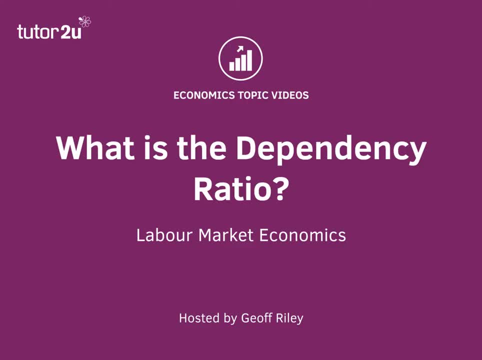 that year is reached, So this has been a short video on the age dependency ratio. 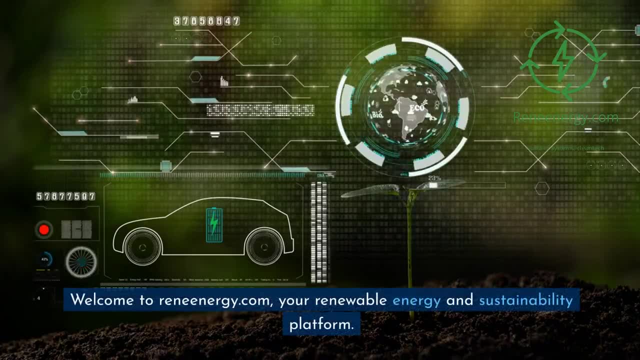 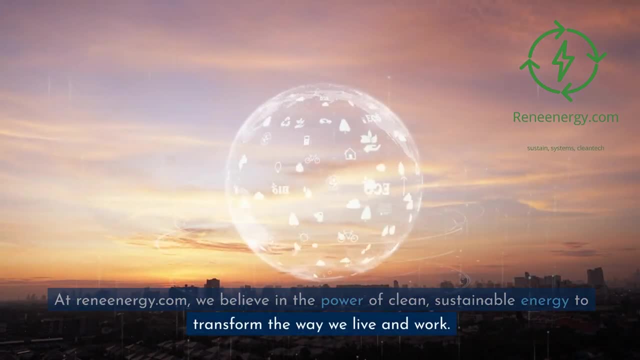 Welcome to ReniEnergycom, your renewable energy and sustainability platform. At ReniEnergycom, we believe in the power of clean, sustainable energy to transform the way we live and work. That's why we offer a range of solutions for businesses and homeowners looking